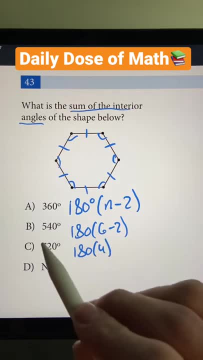 which is 180 times 4,, which is going to be 720 degrees. 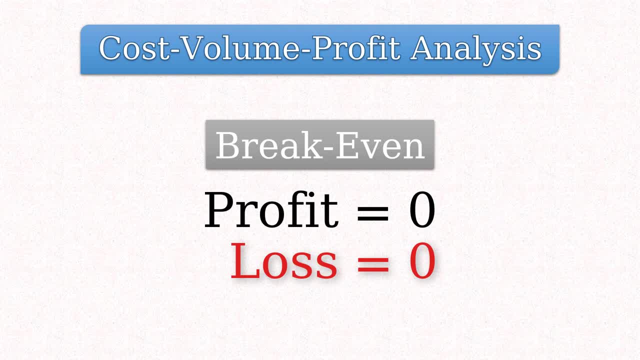 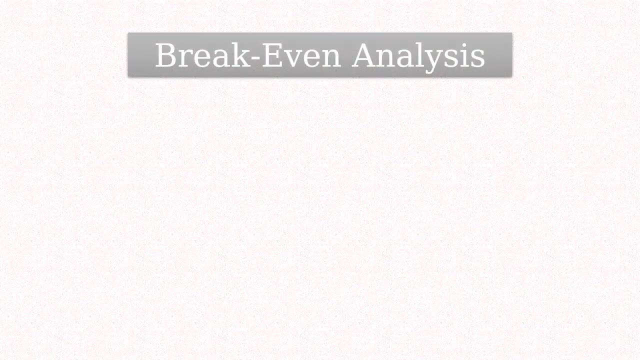 The break-even point refers to the minimum quantity of a product to sell without generating a loss, or how much sales are required before a business starts making profit. So at break-even point total revenue equals total cost. In theory, total cost is divided mainly into fixed costs and variable costs.